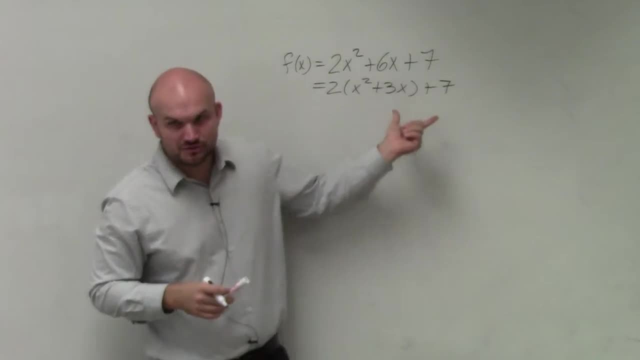 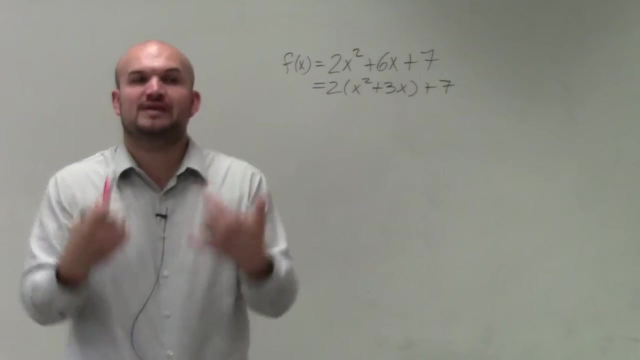 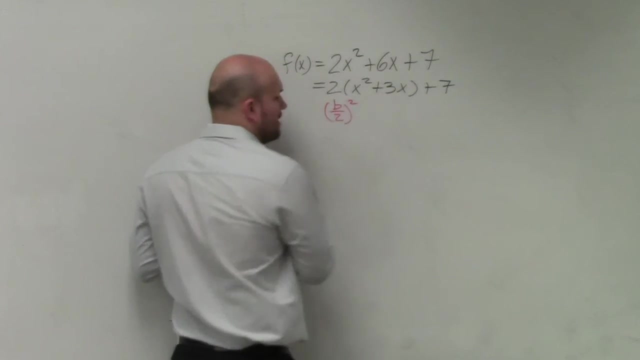 Okay, I'm just going to factor out the first two terms. Now again, the goal of completing the square is to create a perfect square trinomial. So we have to create a perfect square trinomial. To do that, what we do is we take b, divide it by 2, and we square it. b in this case is 3.. So after I factor out the 2,, my b- in my parentheses- is 3.. So what I'll do is I'll take 3, divide it by 2, and square it. 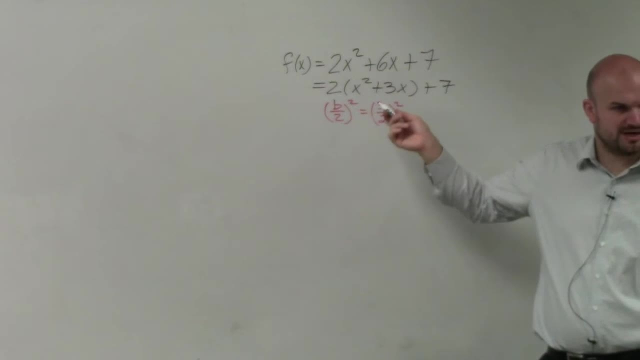 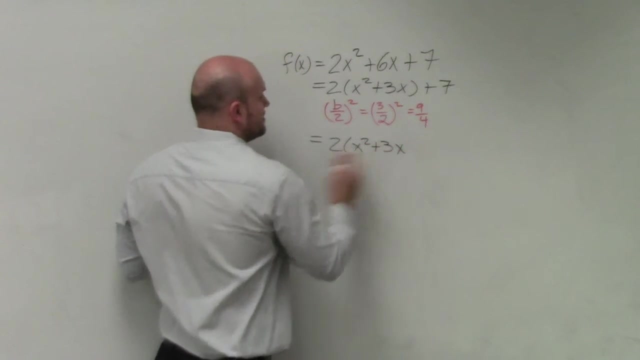 Now 2 doesn't divide into 3 like we've done in these other problems. right, That's okay, We'll just square it and that's going to give us 9 fourths. Now we add the 9 fourths inside the parentheses. and we have to now subtract the 9 fourths outside the parentheses, right, Because you can't just add the number. So we do 2, and we have x squared plus 3x plus 9 fourths. 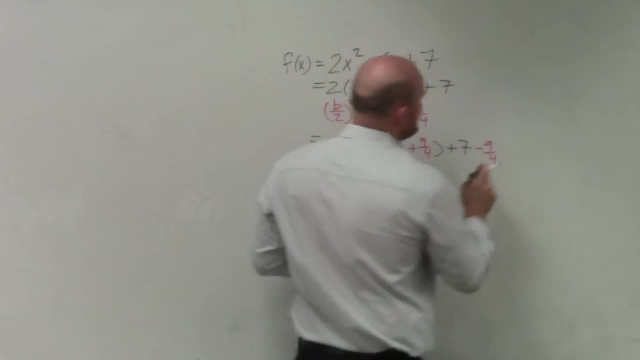 And then minus 9 fourths. But please realize that I'm not adding a 9 fourths. actually I'm adding a 9 fourths that's being multiplied by 2.. So over here I have to multiply a 9 fourths that's being multiplied by 2.. 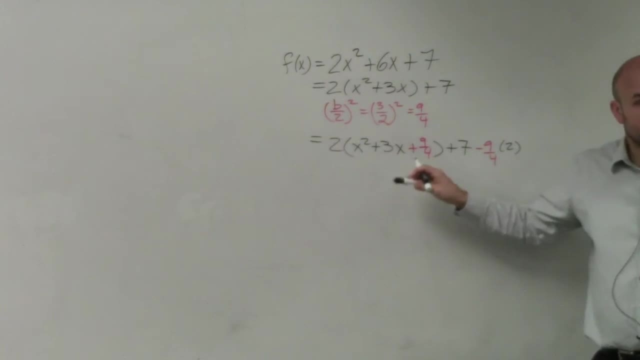 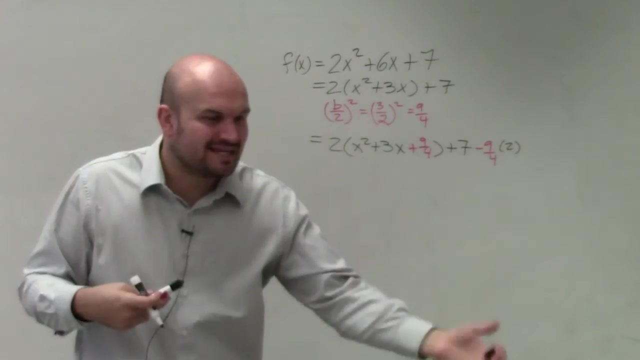 All right. Now, this is a perfect square trinomial. Every single time, ladies and gentlemen, you do complete the square, you create a perfect square trinomial. Unless you're playing on your phone, you might not have a perfect square trinomial. 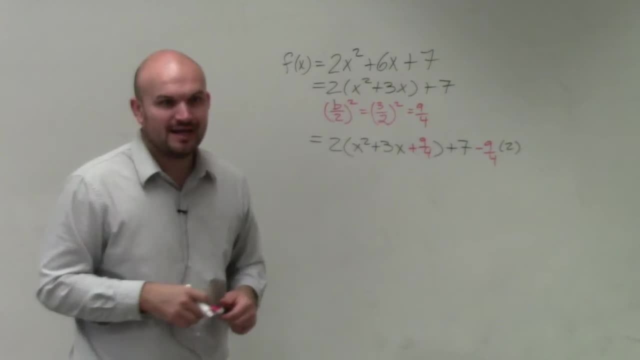 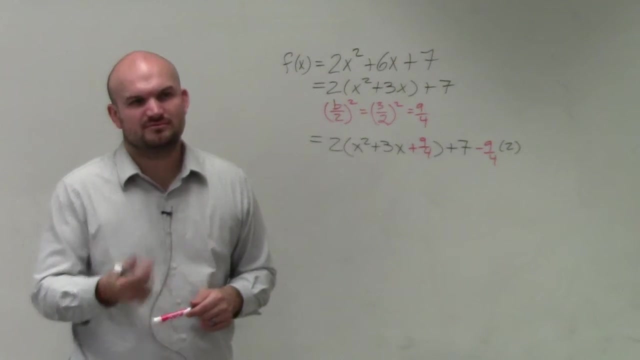 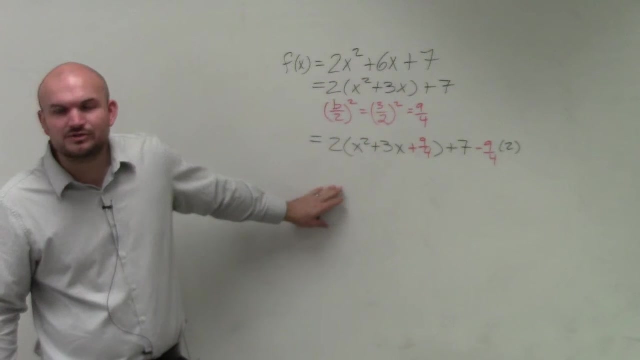 But if you are completing the square, you will create a perfect square trinomial. You will create a perfect square trinomial. Why are perfect square trinomials so helpful? Because they can always be factored down to binomials squared. 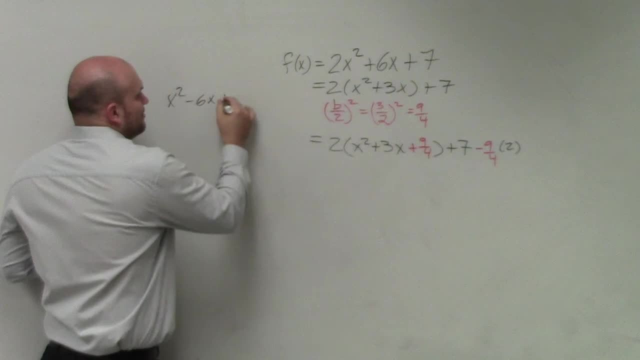 Remember we kind of practiced this Like x squared minus 6x plus 9.. That's a perfect square trinomial. It can be factored down to a binomial squared. Remember we kind of practiced this Like x squared minus 6x plus 9.. That's a perfect square trinomial. It can be factored down to a binomial squared. 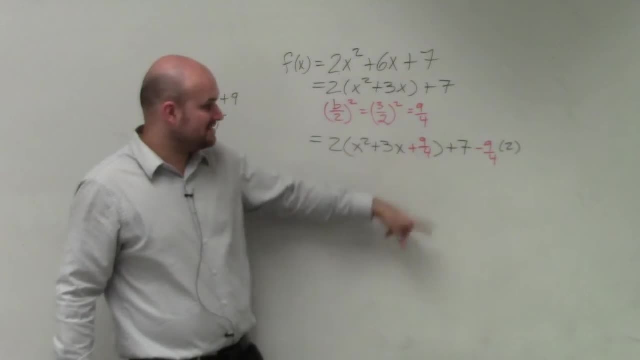 That means there's some number that multiplies by itself to give me this, but then it has to give me 3.. So what number multiplied by itself gives me 9 over 4?? 3, 3 halves, So x plus 3 halves squared.